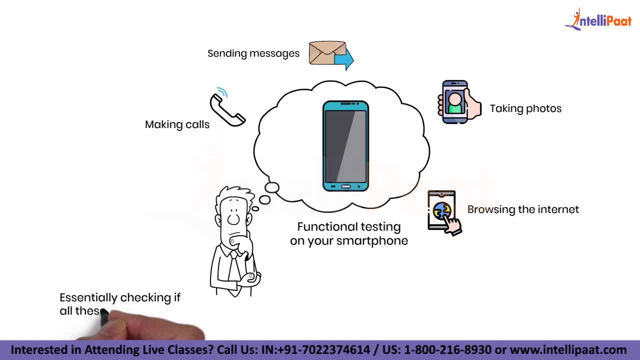 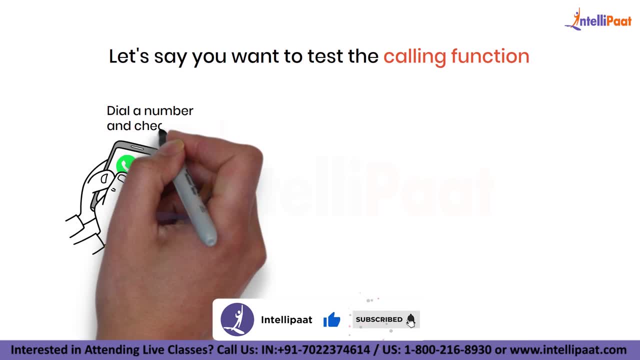 use functional testing on your smartphone. you are essentially checking if all these functions are working correctly. Let's say you want to test the calling function. You would dial the number and check if the call goes through, If you can hear the other person and if they can hear you. 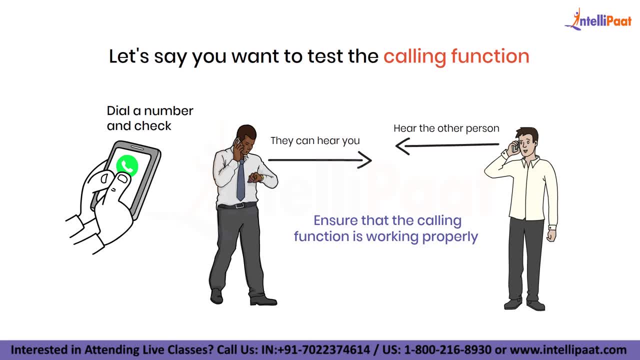 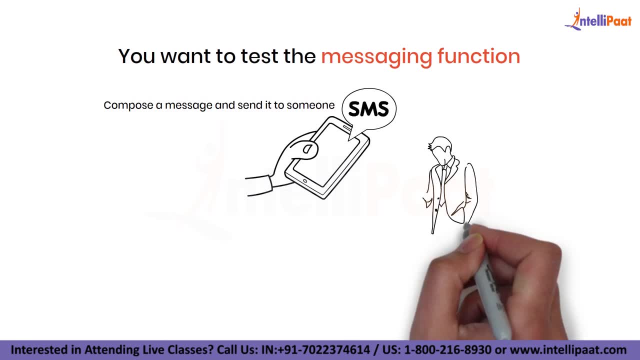 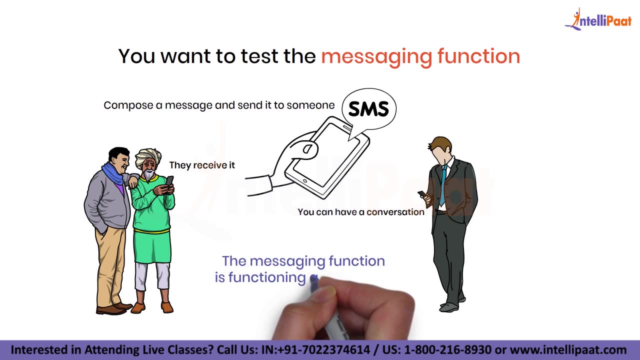 this is to ensure that the calling function is working properly. Suppose next you want to test the messaging function. You would compose a message and send it to someone, thus making sure that they receive it and you can have a conversation. This ensures that the messaging function is functioning as expected. Similarly, you would 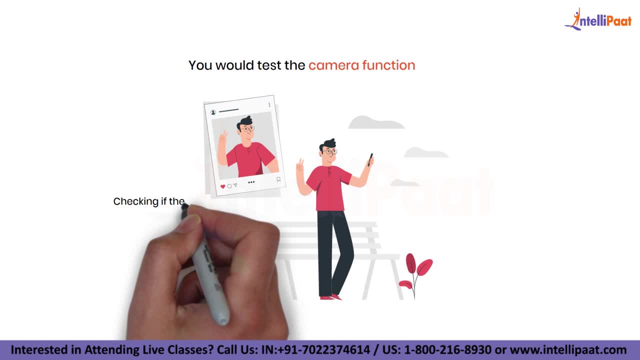 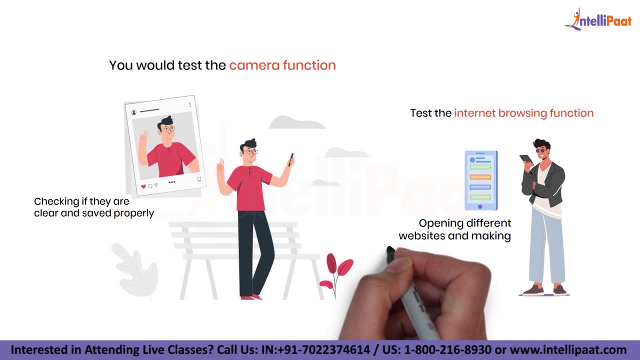 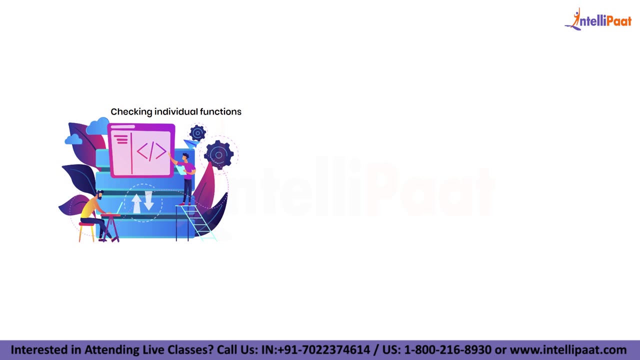 test the camera function by taking photos and checking if they are clear and saved properly. You would also test the internet browsing function by opening different websites and making sure that they load correctly. Functional testing is just not about testing. It's about checking individual functions but also how they work together. for example, you would test if you 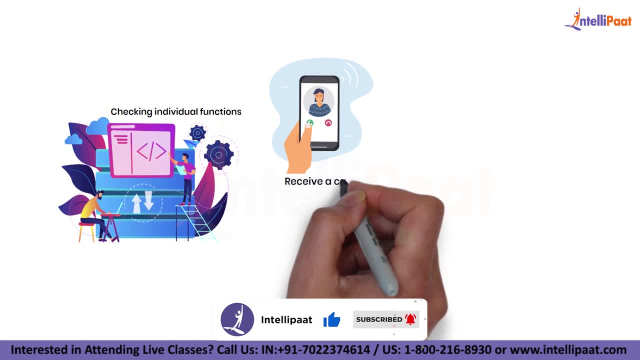 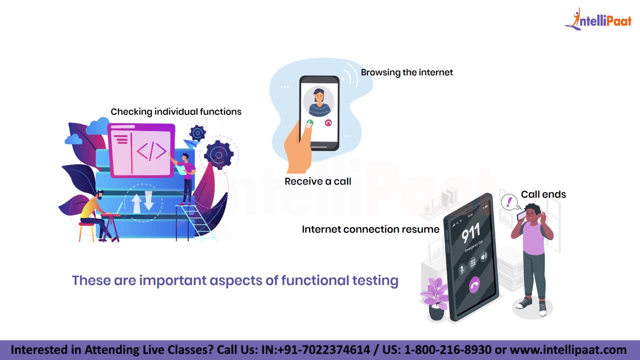 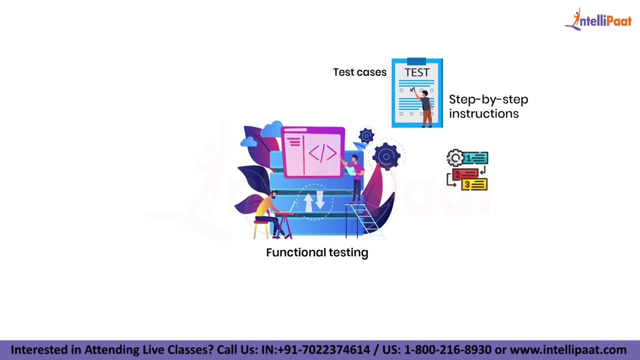 can switch between functions seamlessly. can you receive a call while browsing the internet and does the internet connection resume after the call-ins? these are the important aspects of functional testing. during the functional testing, testers create test cases which are like step-by-step instructions to perform different tasks and validate the expected outcomes. they carefully 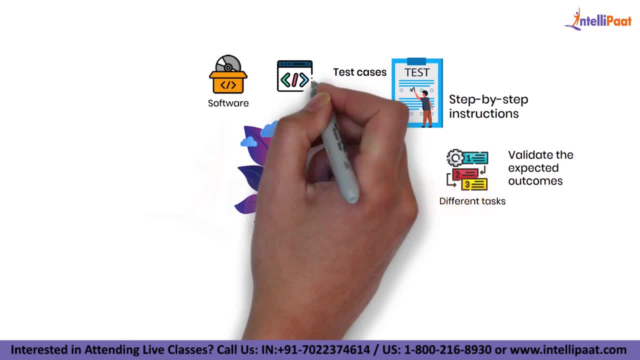 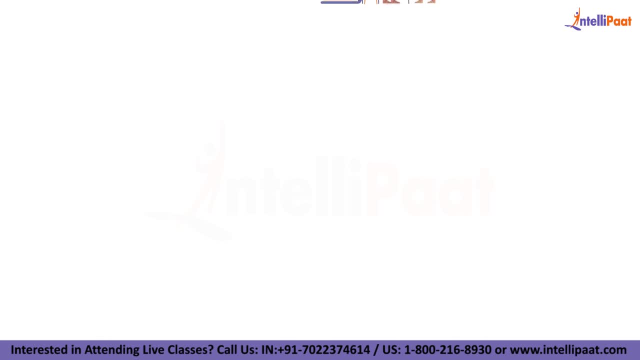 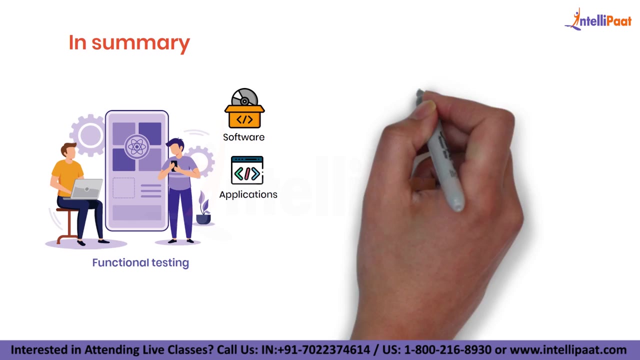 follow these instructions to ensure that the software or application is behaving as intended. if any issues or bugs are found, they are reported to the development team, who then fix them. in summary, functional testing is all about ensuring that the software or applications do what they are supposed to do. it's like checking if all the functions of your smartphone are working. 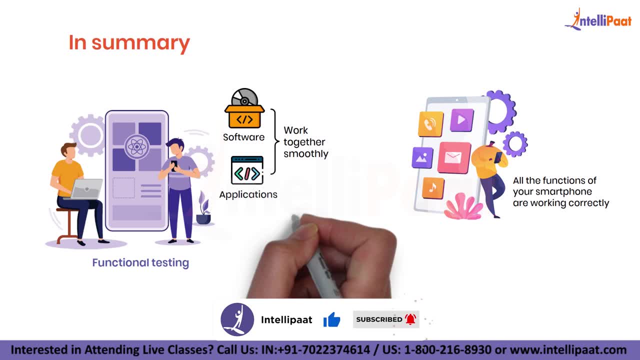 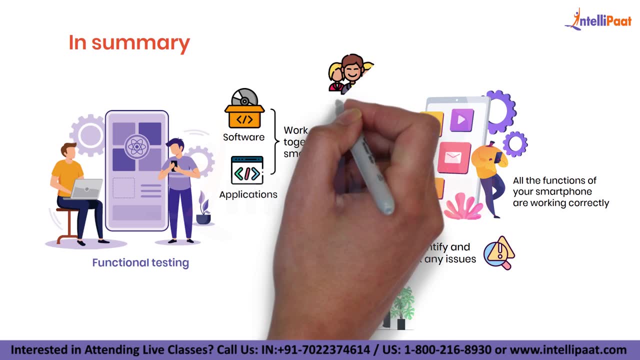 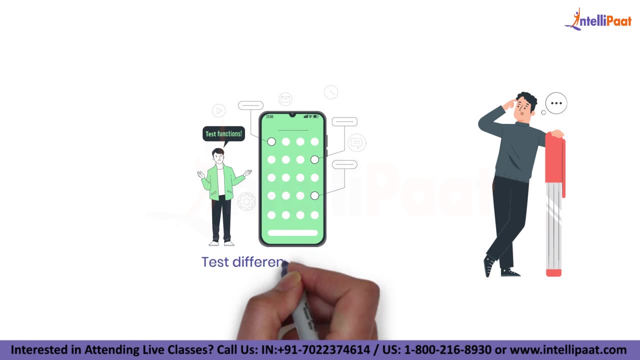 correctly and they work together very smoothly. by conducting functional testing, we can identify and fix any issues before the software or application is released to the users, thus ensuring a better user experience and a reliable product. remember, just like how you test different functions of your smartphone. functional testing: 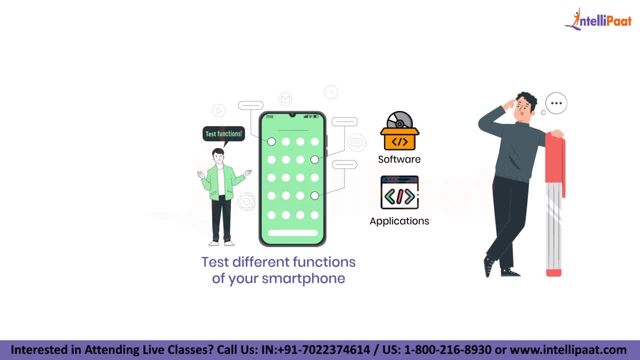 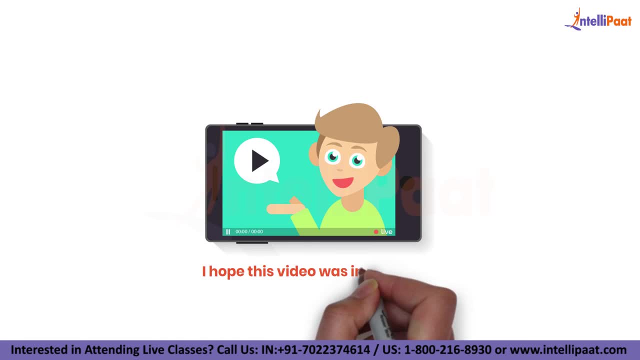 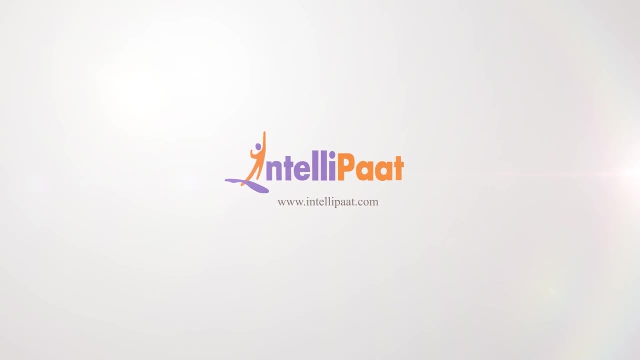 is about checking if software or applications meet their intended purpose and perform their tasks accurately and efficiently. and that's a wrap. i hope this video was informative. to come across more content like this, subscribe to intel part youtube channel and like this video. if you have any questions or comments, please feel free to ask them in the comments section below, and i'll see you in the next video.